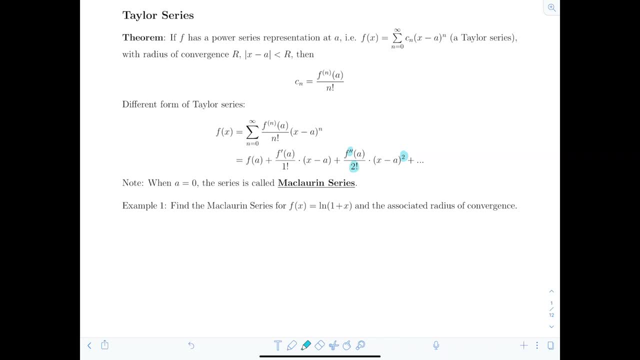 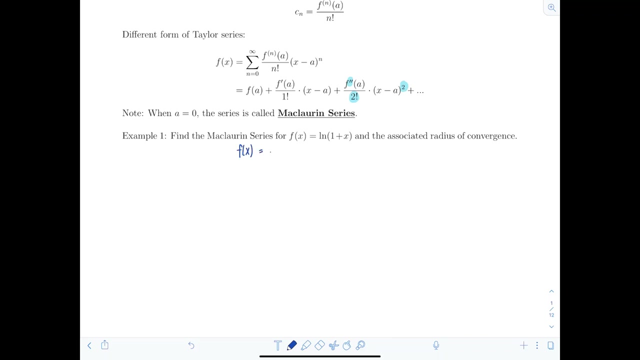 important. Now let's look at an example. So find the McLaurin series for f of x equals the natural log of one plus x and the associated radius of convergence. So we're going to use the formula here. The function f of x is natural log of one plus x. And since they told me to find a McLaurin, 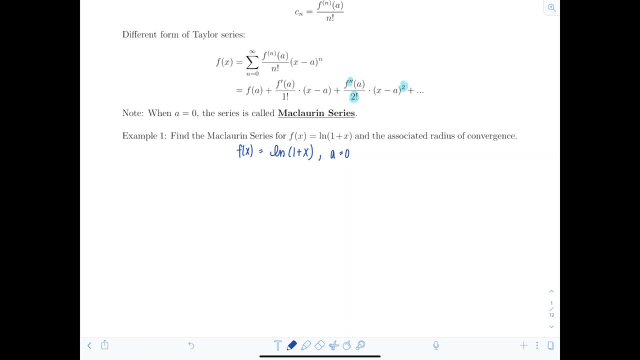 series, I'm going to use the function f of x, And since they told me to find a McLaurin series, then that means a is equal to zero. So how do we begin the process? Well, we need to figure out what the coefficients are, right? So I'm going to compute the nth derivative of my function. 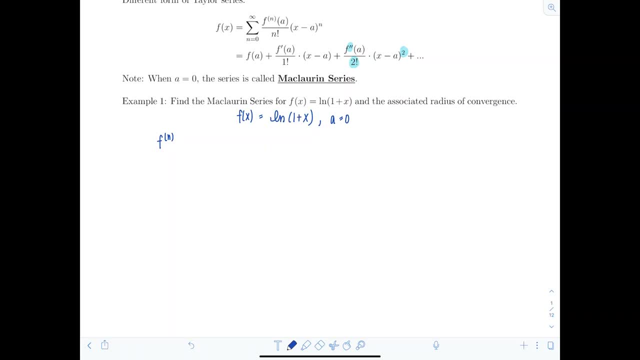 at a or of x for now. Then I'm going to substitute in zero And then I'm going to put it all together and figure out what the coefficient is. So it's going to be the nth derivative at zero divided by n factorial. 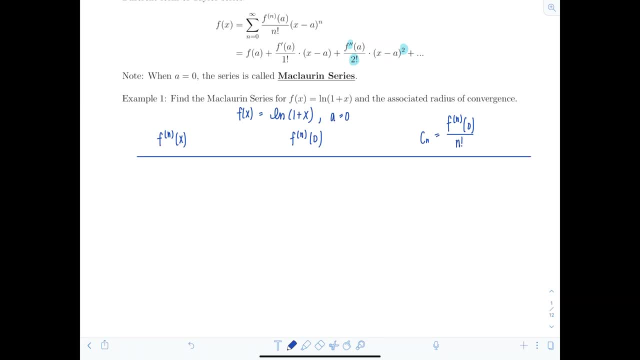 Okay, so let's make a little table, And the process is: you compute enough derivatives, fill this in, build the coefficients until you see a pattern and you can write it in sigma notation. So here we go. We're going to fill in the first column first, So the zeroth derivative. 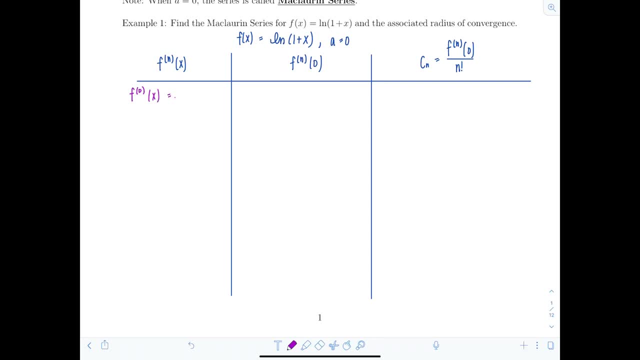 or the original function is just natural log of one plus x. And then the first derivative- we know it's going to be one over One plus x. The second derivative: well, that's one plus x to the negative first. so it's going to be negative one over one plus x squared. The third derivative: 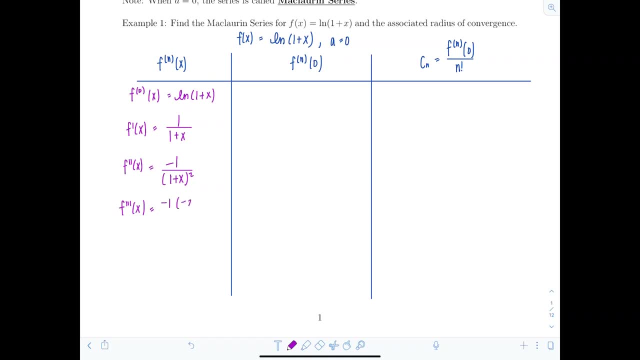 would be negative one times negative, two over one plus x, cubed. And the fourth derivative is going to be negative one times negative, two times negative, three over one plus x to the fourth. I wrote it that way so you could kind of see the pattern that's emerging. Okay, now I'm going to evaluate. 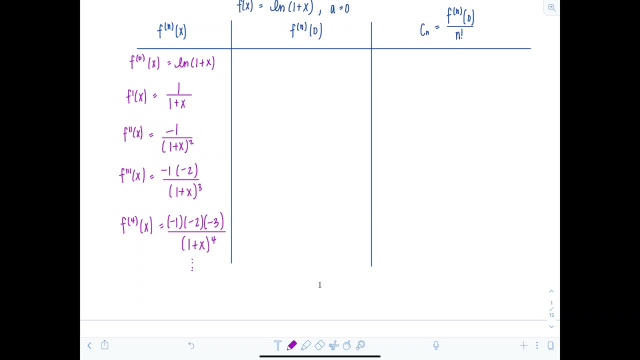 each of these derivatives specifically at zero. Since we're finding a McLaurin series, a is equal to zero. So natural log of one, that's zero. One over one plus zero, that's one. I'm going to have negative, one over one. 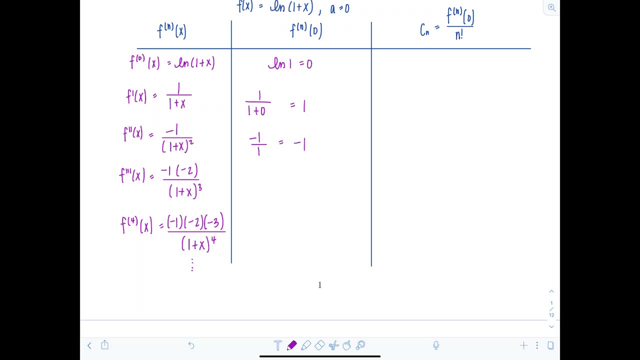 Which is negative one. This is going to be positive two over one which is positive two. This is going to give me negative six over one which is negative six. So notice it's alternating. And then what would the overall coefficients be? So you're going to have this value. 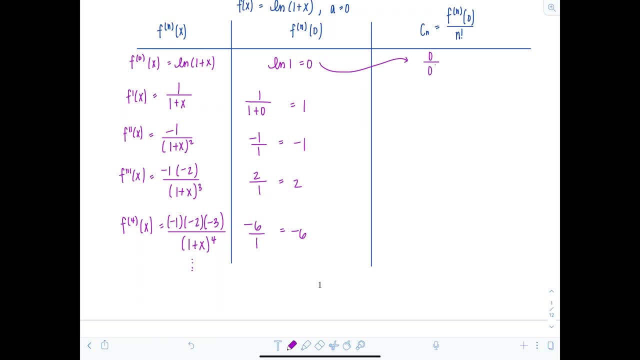 and then just put it over n factorial. So zero over zero factorial. that would be zero. Then we have one over one factorial. This would be negative. one over two factorial. Two over three factorial. Negative. six over four factorial. Okay, so let's see What are we going to be left with here now? I want to put everything all together. 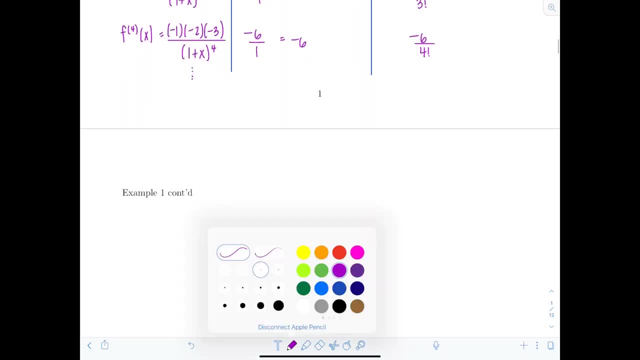 and list out the first few terms. So my function, which is natural log of one plus x, The first term is zero over zero factorial times x to the zero Plus. then I have one over one factorial times x to the first Plus. then the next term is negative, one over two factorial. 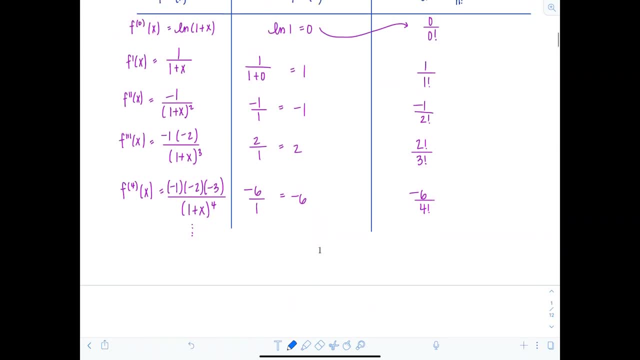 times x squared right. x minus zero squared. I'm getting all of these values from here. Then I'm going to have what's next: Plus two over three factorial times x cubed, plus negative six over four factorial times x. plus three factorial times x cubed. 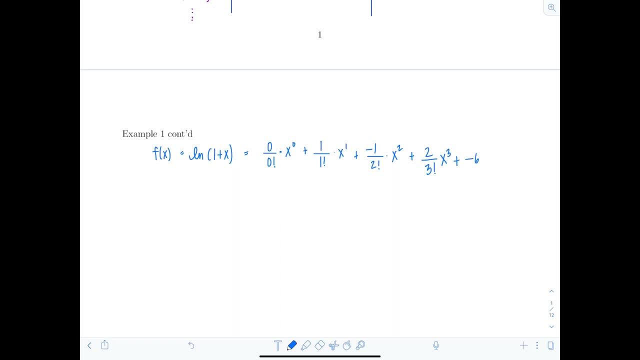 and then final with this force fluid equation. I'm going to take negative two over x factorial. That would be equal to x squared plus negativeと Negative two over two factorial times y squared Or negative to. That would be way better, wouldn't it? 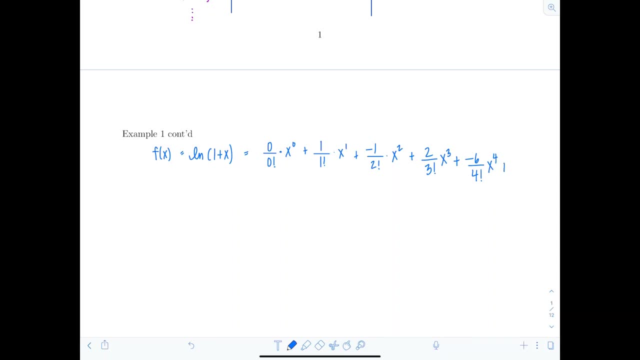 All right, so I'm going to take negative two over three. factorial times x squared first, what do I have? factorial times x to the fourth plus so on and so forth. Okay, Now can we clean up a little bit? Well, let's see, here This first term: this is just zero. so that's gone. Then here, this is just one. 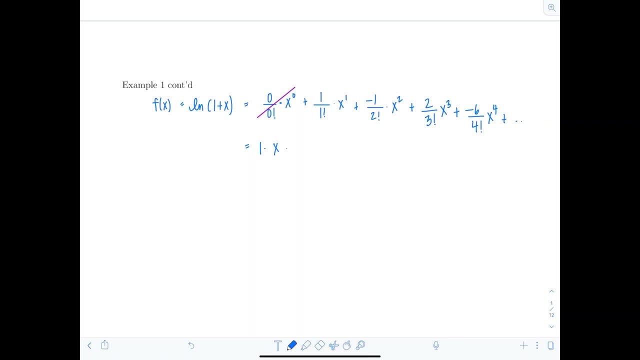 times x to the first. Then I have negative one over two x squared plus two over three factorial. The two is going to cancel out, so I just have one over three x cubed. Four factorial is four times three times two, so the three and the two is going to cancel with the six, so I have minus. 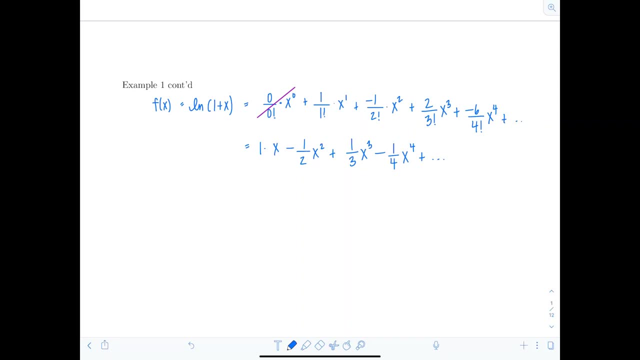 one-fourth, x to the fourth, etc. Hmm, so this looks like a pretty simple pattern, right? I could write this as the sum starting at one going to infinity. Notice, I always have n in the denominator. It's alternating right, And I want the first term to be positive, so I'm going to have negative one. 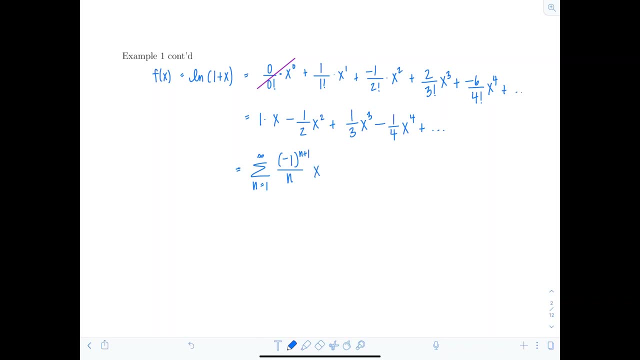 to the n plus one, and then x is raised to the nth power. All right, so there is all of that. So I'm going to write this as the sum starting at one going to infinity. All right, so there is all of that. So I'm going to write this as the sum starting at one going to infinity. 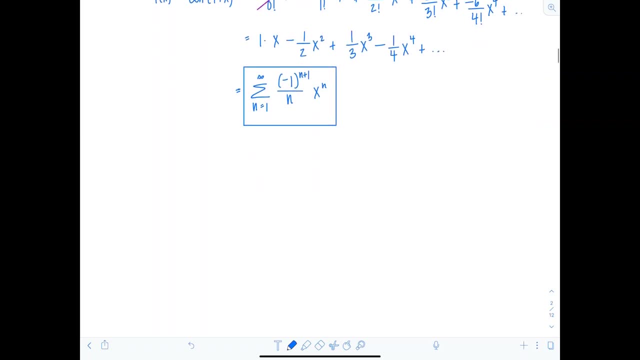 R McLaurin series. Now we need to find the radius of convergence. So how do we do that? Well, in this case I'm going to use the ratio test. so I need to limit as n approaches infinity, absolute value. I'm just going to throw out. 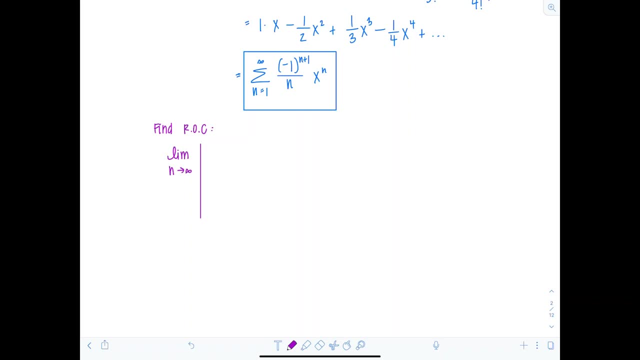 the negative one to the n plus one portion, since I'm taking the absolute value. So I'm going to have x to the n plus one over n, plus one over x to the n over n, which is going to give me the limit as n approaches infinity. 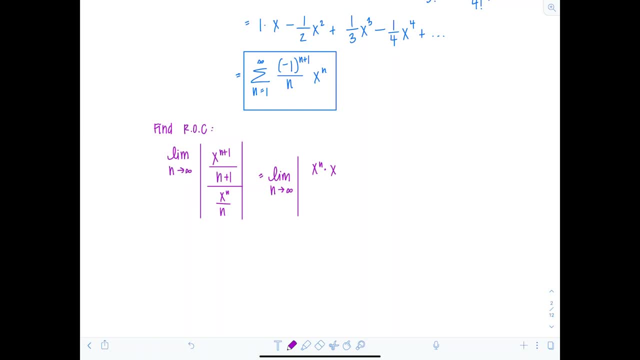 And here we have x to the n times x over n, plus 1 times n over x to the n. Okay, so that x to the n cancels out, and then I can take the absolute value of x outside the limit, right. 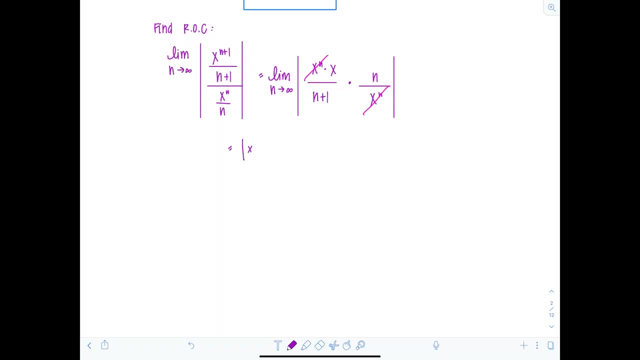 since the limit is as n is approaching infinity, So I can write this as the absolute value of x times the limit as n approaches infinity of n over n plus 1.. As n approaches infinity, n over n plus 1 is going to approach 1.. 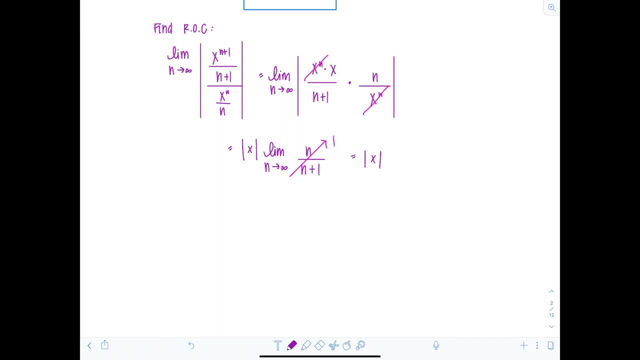 So this limit is equal to the absolute value of x, Which I set strictly less than 1.. So what does that tell me? My radius of convergence is equal to 1.. All right, good, Let's look at another example, this time centering it somewhere else. 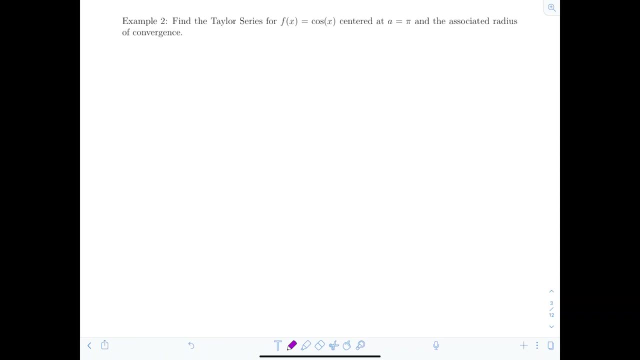 So here in example 2, we're going to find the Taylor series for f of x, equals cosine of x, centered at a equals pi, And the associated radius of convergence. So we'll make the same sort of table. here We're going to have the nth derivative of our function. 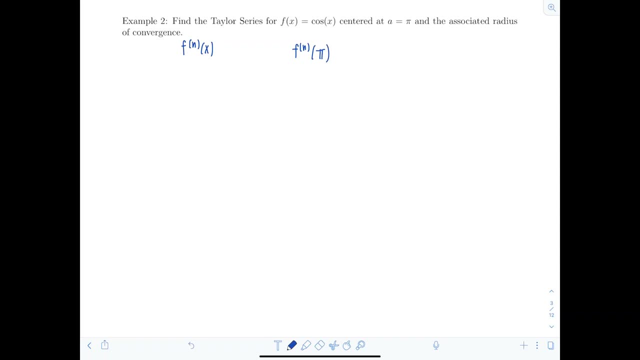 the nth derivative evaluated at pi, and then the coefficient. So we'll have the nth derivative at pi, remember, divided by n, factorial, And just do enough until you see a pattern. So sometimes it'll take more derivatives for certain functions than others, depending. 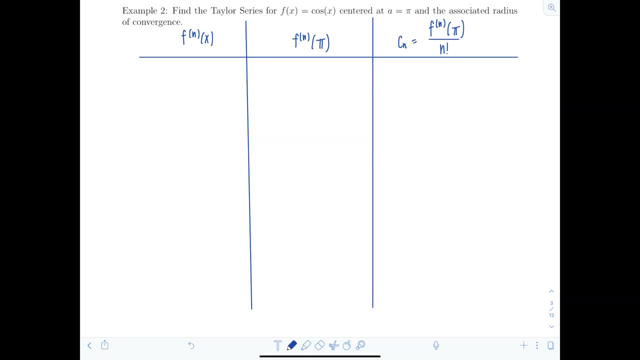 Okay, I'm going to take about six derivatives, just in case you want to know how far to make your table. So the 0th derivative, or the original function, is cosine of x. First derivative is negative sine x. Second derivative: keep the negative cosine x. 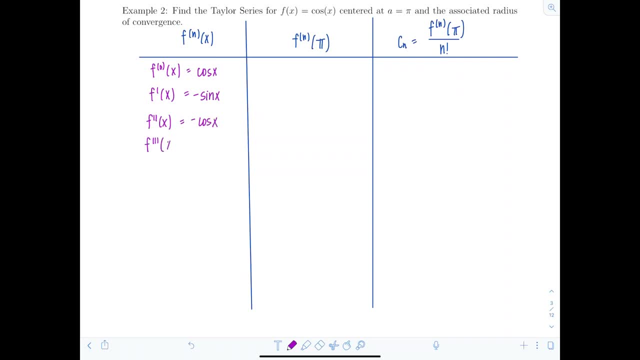 Third derivative is sine x. And then fourth derivative gives us back cosine x. right, The derivatives are on a cycle of length. four Fifth derivative- why not? We already have it. you can just copy from the first Negative, sine x. 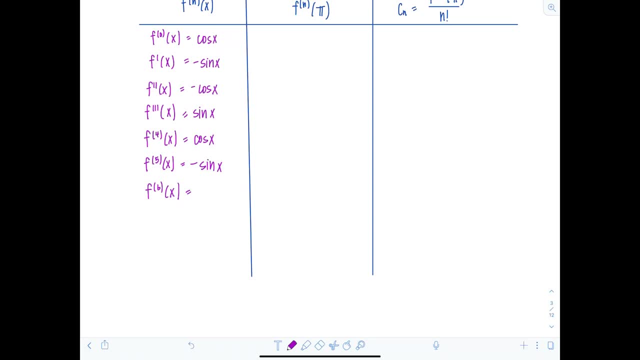 Sixth derivative is going to match with the second, So negative: cosine x, et cetera. Okay, that was a little too much, let's get rid of that. Okay, now let's evaluate these derivatives at pi. So cosine of pi, that's negative one. 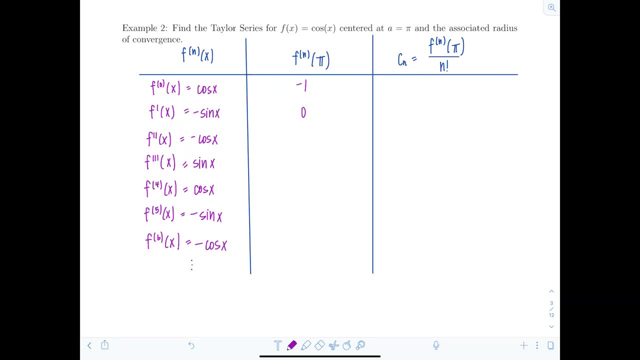 Negative sine of pi is going to be zero, Negative cosine of pi is going to be one, Then we get zero again. So it repeats: Negative one zero, one zero, et cetera. Now what if I divide these by n? factorial: 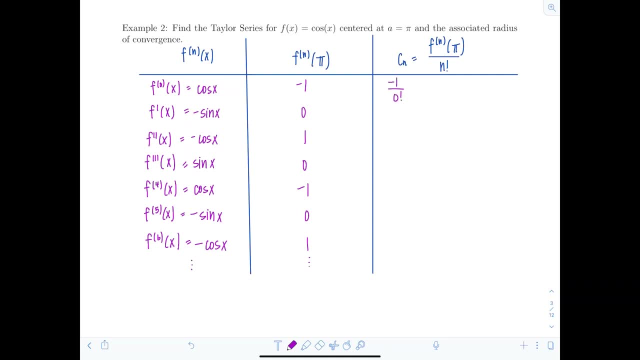 So I'm going to do that. So I'm going to have negative one over zero factorial, which is one. So this would be negative one. Zero divided by any non-zero number is zero. Then I'm going to have one over two factorial zero. 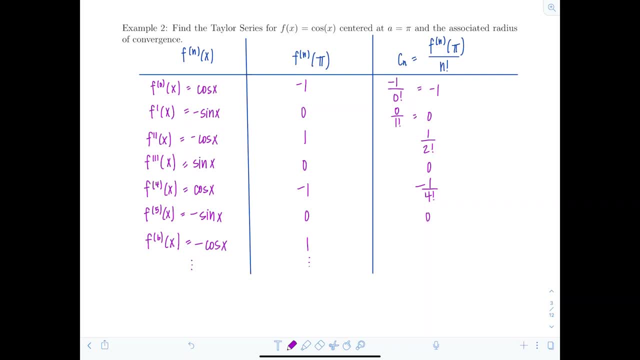 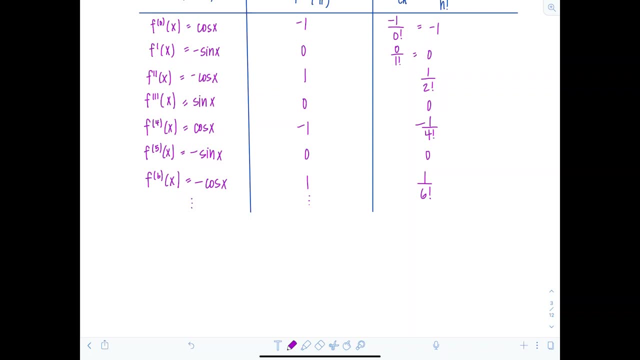 Negative one over four factorial. zero. Positive one over six factorial, And then we'd get a zero. Okay, so it looks like we're losing quite a few terms here. That's why I took so many derivatives, So let's start listing them out. 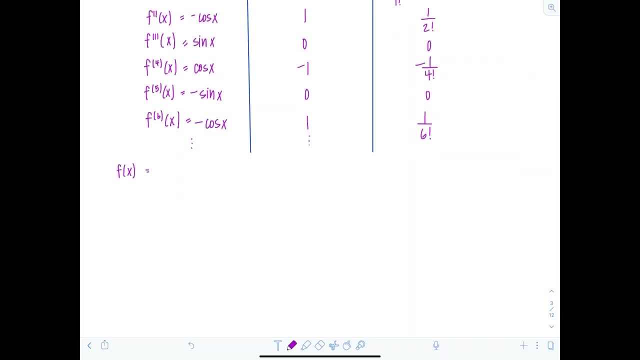 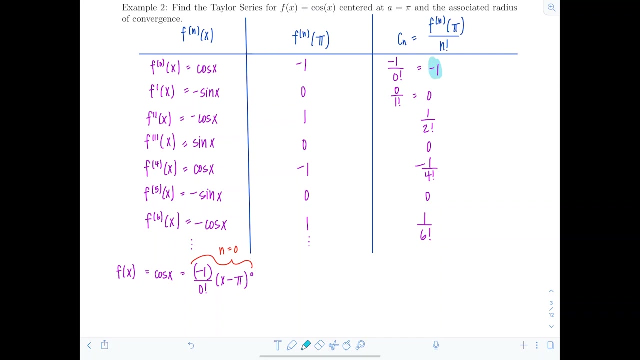 Okay, so f of x, which is cosine of x, is equal to. so the first term was negative one over zero. factorial times: x minus pi to the zero. Now this is for: n equals zero. That's from this guy right here. 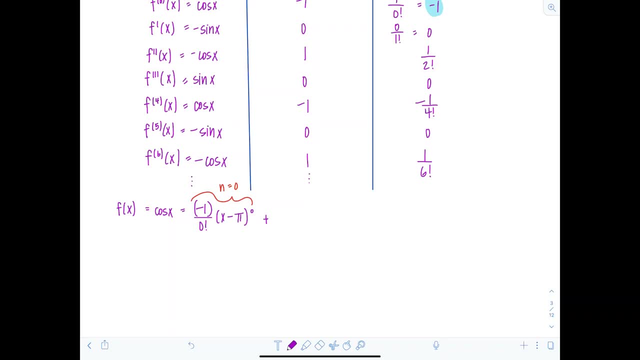 Plus, if n is equal to one, I just get zero. Okay, Plus I'm going to have one over two factorial times x minus pi. squared, That's for n equals two Plus zero, Plus negative one over four. factorial x minus four. 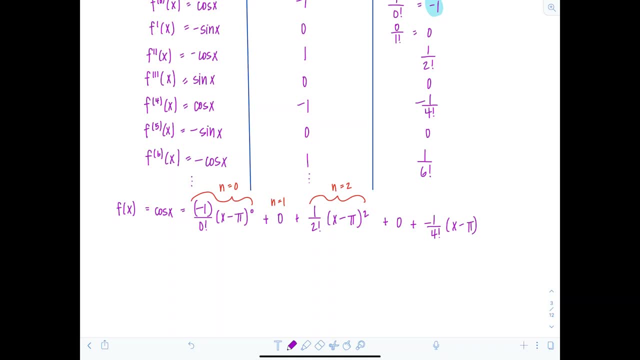 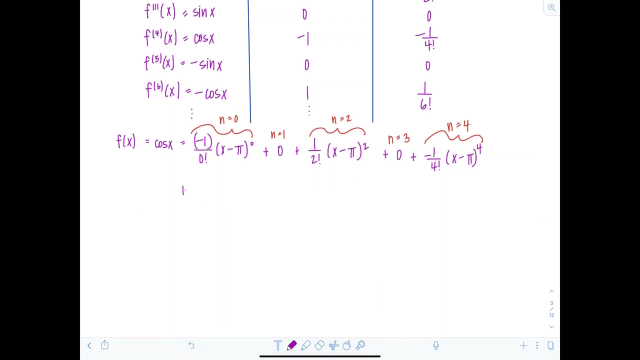 x minus pi, excuse me, to the fourth. So this is n equals three, This is n equals four. Okay, let's keep going. We did more work than that. Plus zero for n equals five Plus one sixth, one over six factorial times: x minus pi to the sixth. 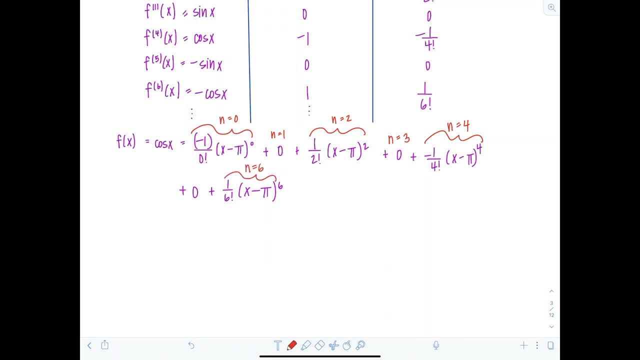 That's for n equals six. This is for n equals five plus dot dot dot. Now notice only the even terms, the terms with an even index, survive right. So this is gone, this is gone, this is gone. 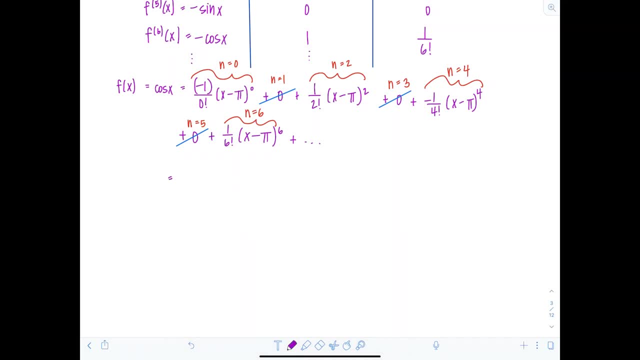 So now I have negative one over zero factorial. I know that's just negative one, but I'm leaving it like that So we can write the pattern out in summation notation. Okay, Times x minus pi to the zero. Then what's the next survivor? 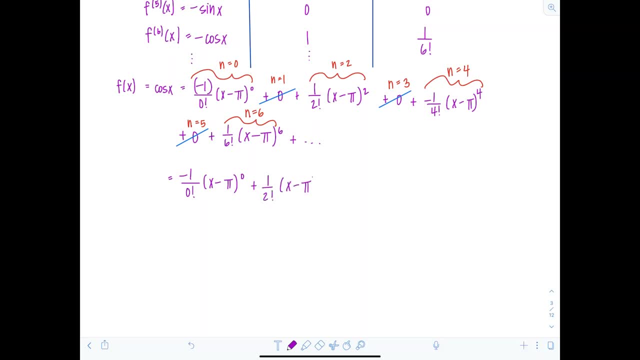 One over two factorial times x minus pi. squared Next, survivor is negative: one over four factorial times x minus pi to the fourth. Then I have plus one over six factorial times x minus pi to the sixth, et cetera. So now I want you to think of this as your new series. 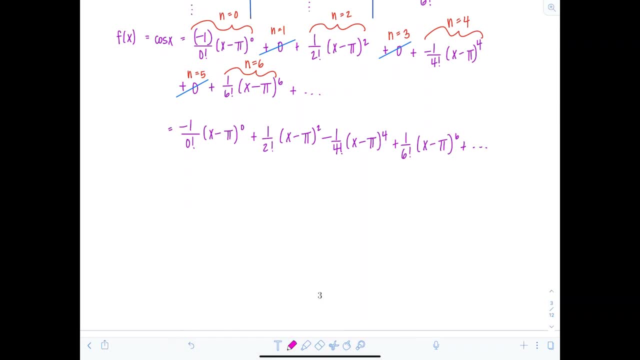 Okay, And we could start writing in summation notation: nicely if I start at zero, right, And then this would be where n is one, n is two, n is three. Okay, So I would write that as the sum n equals zero to infinity. 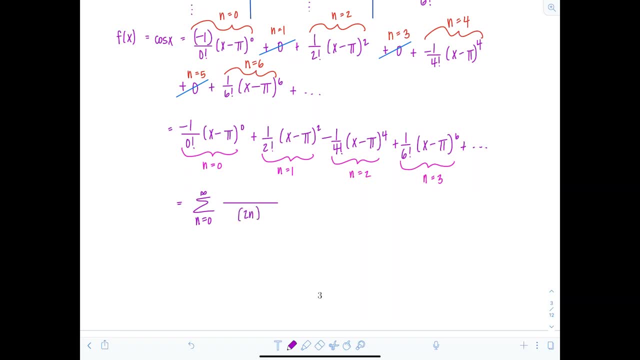 Notice in the denominator. I have two n factorial Right. Since they're all even factorials, I'm gonna have x minus pi raised to the two n even exponents on all of those, And then I need the first term to come out to be negative. 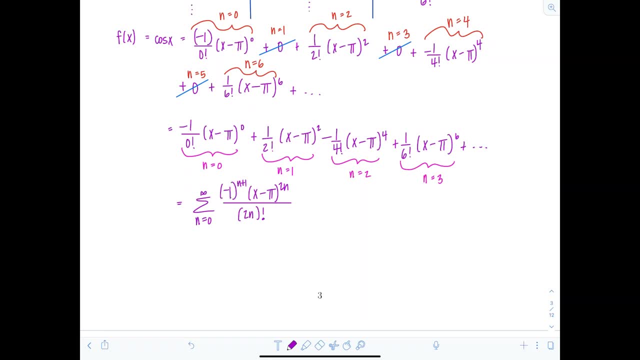 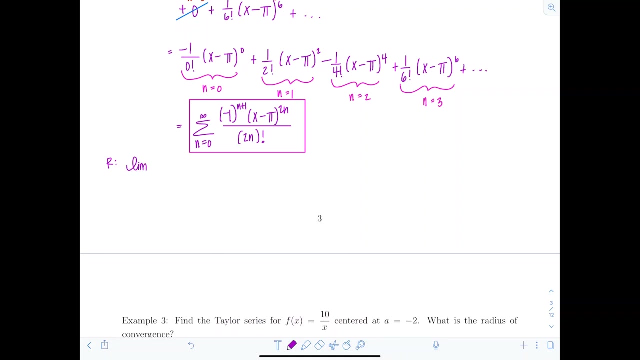 So I want negative one to the n plus one. So there we go. And then now we need to find the radius of convergence. So again, we're just gonna use the ratio test. So I'm gonna look at the limit as n approaches infinity. 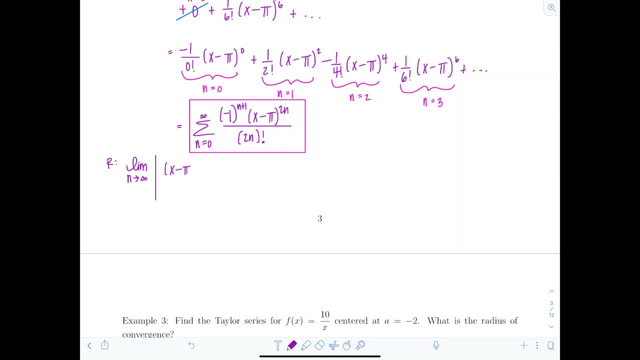 absolute value. I have x minus pi. I'm already gonna substitute in two times n plus one over. this is gonna be two times n plus one factorial, And then let's just go ahead and multiply by two n factorial over x minus pi to the two n. 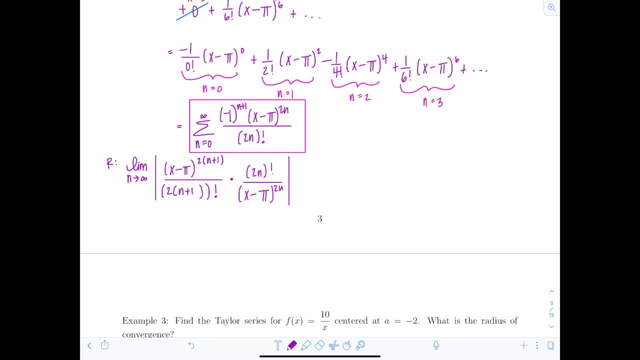 I have absolute value of all of that. And then this is gonna give me the limit as n approaches infinity. Now the exponent would be two n plus two. So I'm just gonna have x minus pi squared leftover, And then over here we have two n plus two factorial. 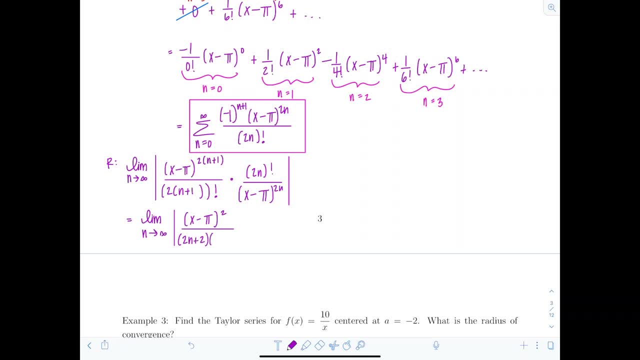 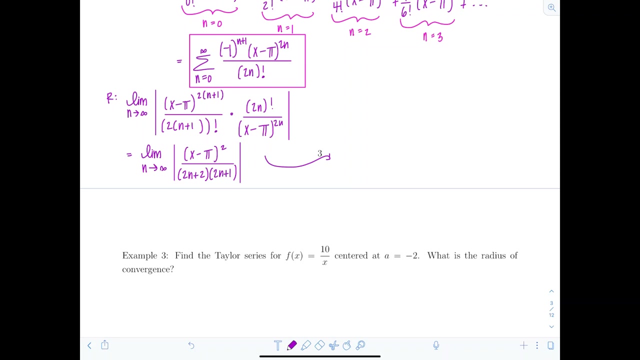 So that'll cancel with the two n factorial, but I'll have two n plus two and two n plus one leftover. Okay, I can take that x minus pi squared outside the limit And I don't need the absolute value, since that's not ever gonna be negative. 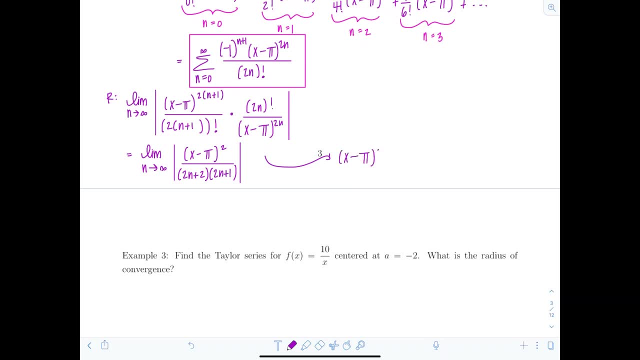 So I have x minus pi squared times the limit, as n approaches infinity, of one over two, n plus two times two n plus one. And as n approaches infinity approaches infinity, this quantity goes to zero. so this limit is actually going to be zero, which is always less than one. so what does that mean? my radius of 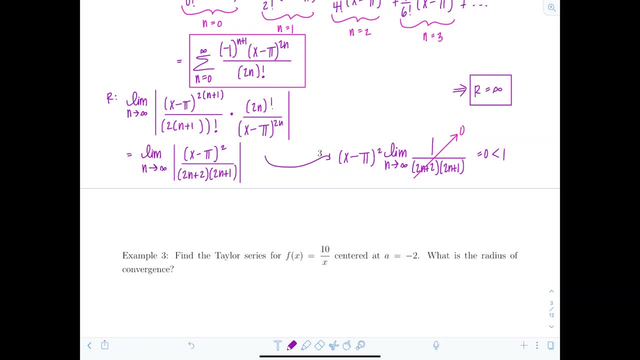 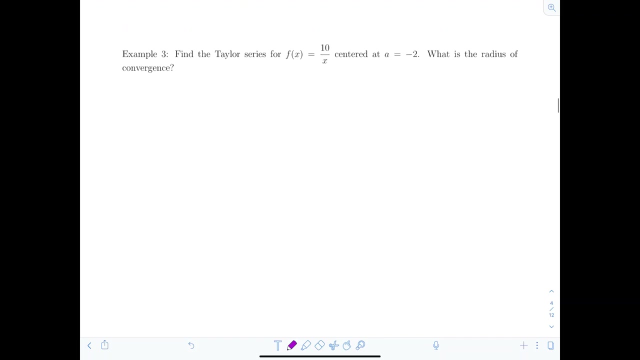 convergence is infinity, infinite. all right, that's a good one. one last example. so find the Taylor series for f of X equals 10 over X, centered at a equals negative 2, and then what is the radius of convergence? okay, so here we go, we'll make our table again. in fact, we can just kind of get going with this one, I think. 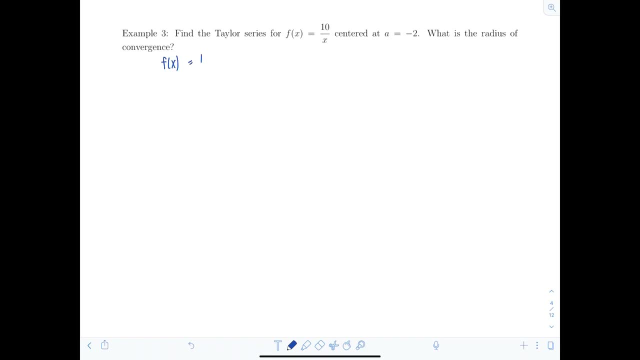 we're professional now. so we have: f of X is 10 over X. so f prime of X is going to be 10 times negative 1 over x square. f. double prime of X is going to be 10 times negative, 1 times negative, 2 over executed, do you? 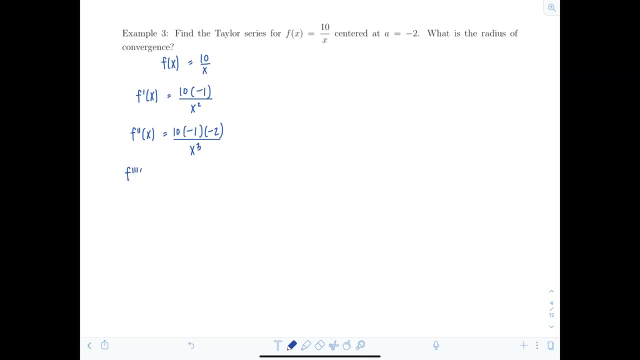 notice a pattern a little bit. f triple prime of X is gonna be 10 times negative, 2 negative, 1 times negative, 2 times negative, 3 over X. to the fourth. do you feel a factorial coming on? and then fourth derivative is 10 times negative. 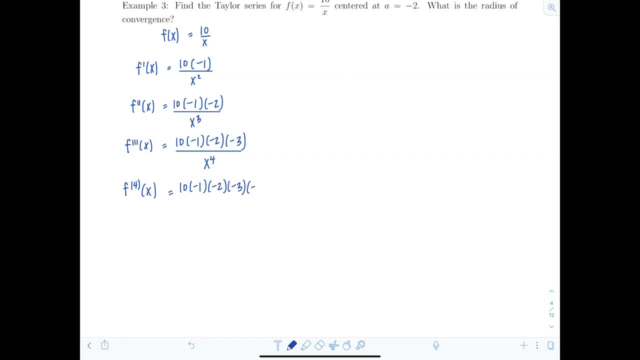 1 times negative, 2 times negative, 3 times negative, 4 over X to the fifth, etc. now I'm gonna substitute in negative 2 for a, so f of negative 2, that's going to be negative 10 divided by 2. I'm just going to leave it like that for second. 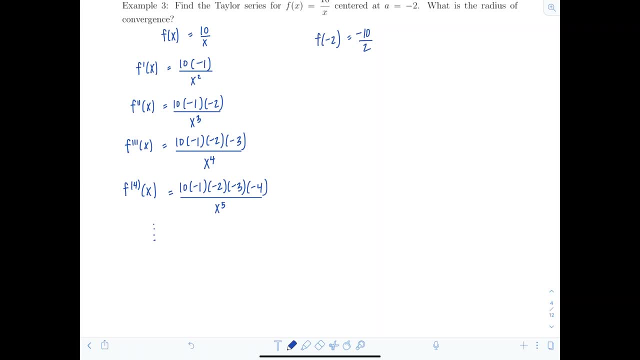 and then let's see what else we have here. so f? prime of negative 2: that's going to be negative 10 times 1 over 2 squared. F double prime of negative 2 is going to be: let's see, negative, right, Because 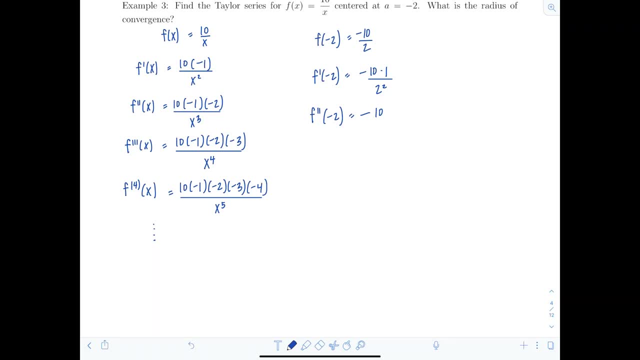 I'm going to cube it. so there's still going to be a negative 10 times 1 times 2 over 2 cubed F, triple prime of negative 2, that one's also going to be negative. So negative 10 times 1 times 2. 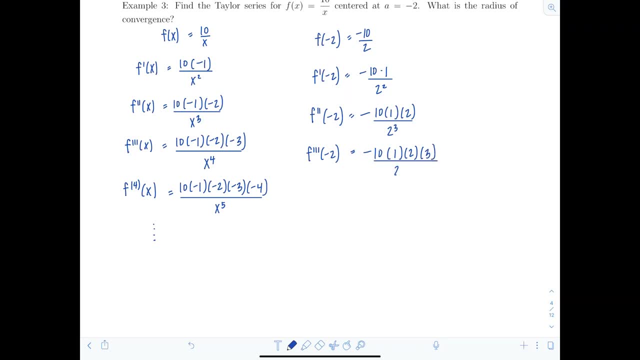 times 3 over 2 to the fourth. Let's do the last one. So the fourth derivative evaluated at negative 2, this one's also negative 10 times 1 times 2 times 3 times 4 over 2 to the fifth. So notice, 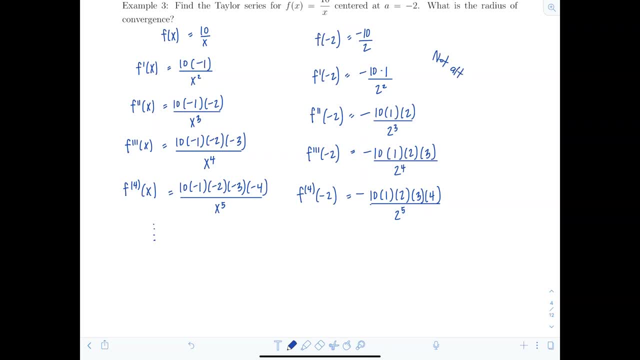 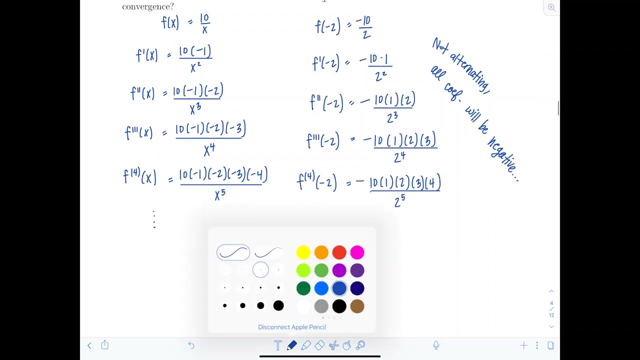 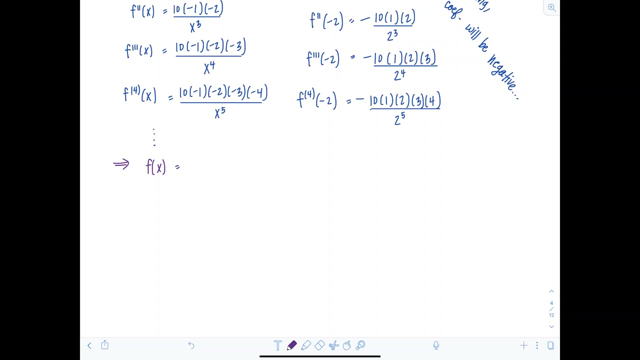 this is not alternating. All the coefficients will be negative, So keep that in mind. Okay, so now let's start writing out the first few terms of our Taylor series. So f of x, which is 10 over x, I can write it as negative: 10 over x. 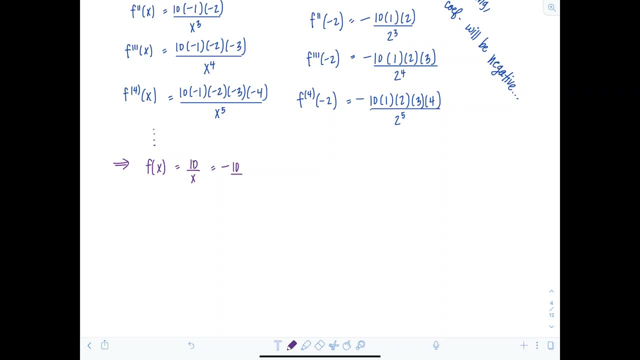 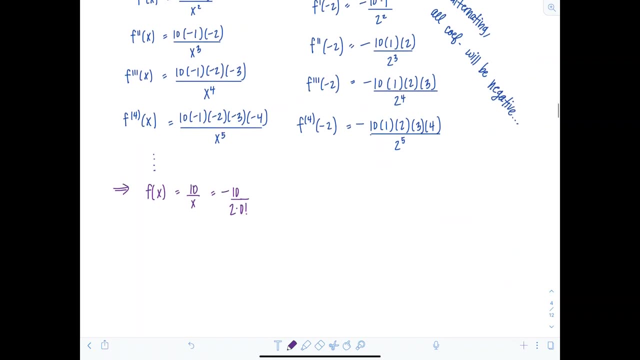 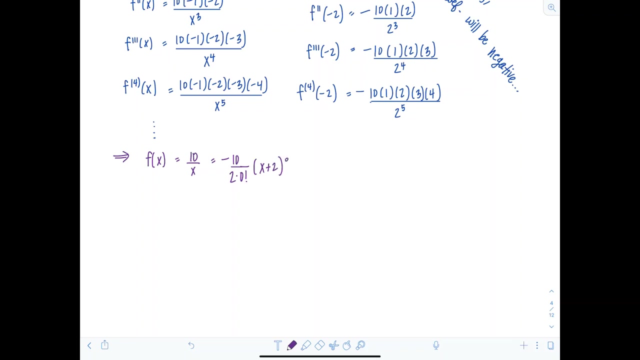 10 over 2, put a 0 factorial there, right? So I took my original coefficient, just threw a 0 factorial in the denominator and then I have x minus negative 2, so x plus 2 to the 0. Okay, next term also negative. 10 times 1 over 2. squared times 1 factorial times x plus 2. 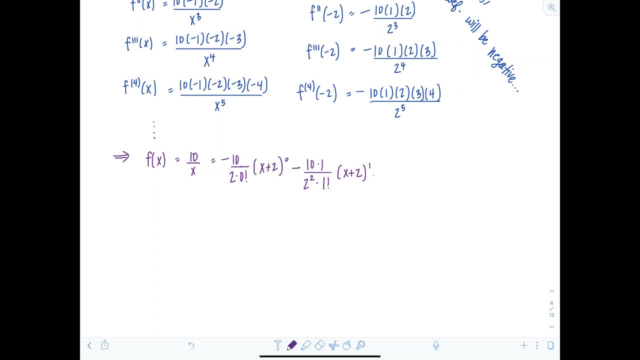 to the first Next term. minus this is 10, times 1 times 2, that's 2 factorial right Over 2 cubed. and then I have 2 factorial times x plus 2 squared, minus 10 times 1 times 2 times 3, that's 3 factorial over 2 to the fourth times 2 squared. 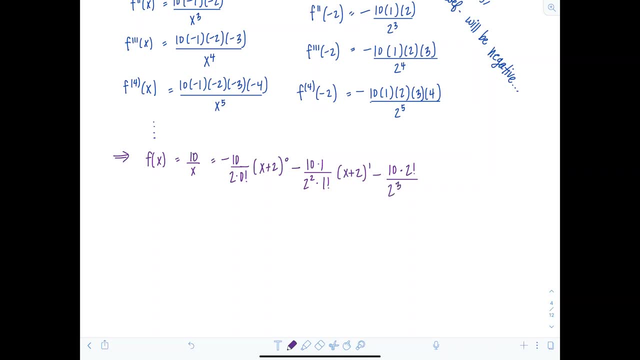 Over 2 cubed. and then I have 2 factorial times x plus 2, squared minus 10 times 1 times 2 times 3, that's 3 factorial Elvis 1 times 2 times 6 times 3 factorial times x plus 2 cubed, etc. 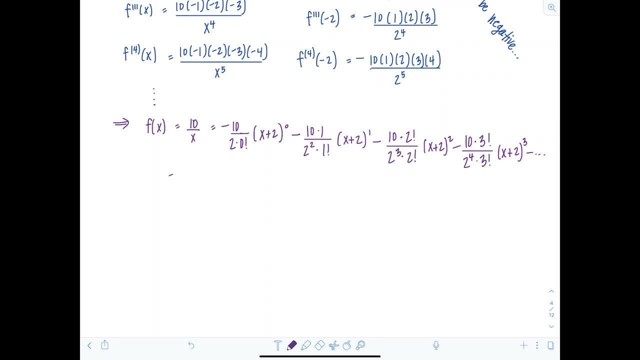 So look, we can clean thisi up a little bit. I can write this as negative 10 over. we'll just leave it like this: 2 times 0, factorial times x plus 2 to the 0. But the factorial can cancel out: right, These cancel, these cancel, these cancel. So really. 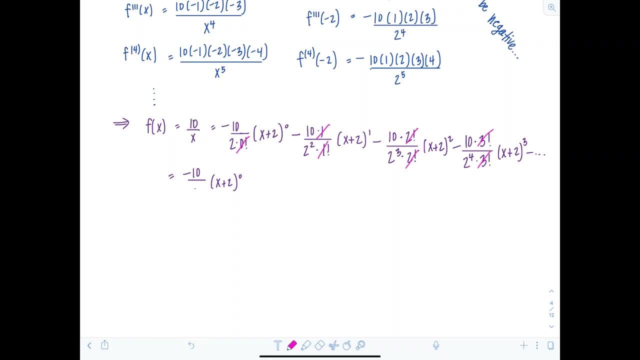 I don't even need this anymore. It's not going to remain in any of the terms, So I'm just going to leave that as a 2.. Then the next term I can write it as negative: 10 over 2 squared times x plus 2 to the first, minus 10 over 2 cubed times x plus 2 squared minus 10 over. 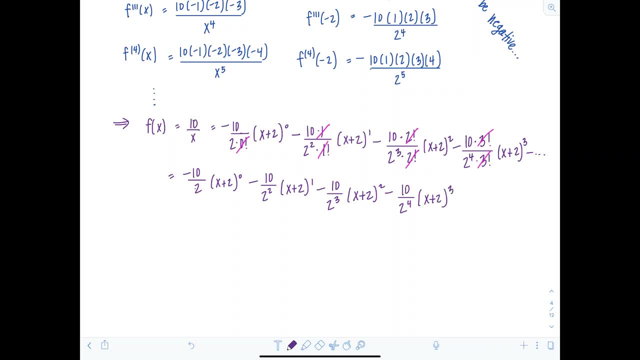 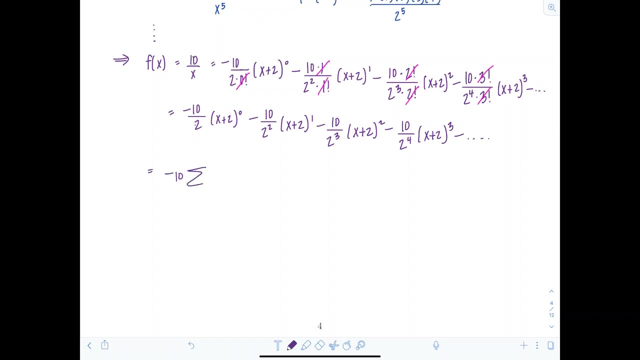 2 to the fourth times x plus 2, cubed minus, et cetera. So do you see a pattern? Well, I see a negative 10.. I'm just going to leave that outside. the sum We can start at n equals 0 to infinity, And then notice, x plus 2 is raised to the n. 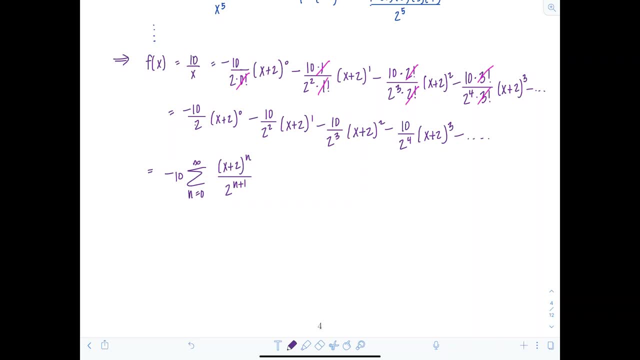 but 2 is raised to 1 power higher. 2 is raised to the n plus 1.. OK, that looks good. Now can we clean this up a little bit? OK, so I can write the denominator. This is negative 10 times the sum. 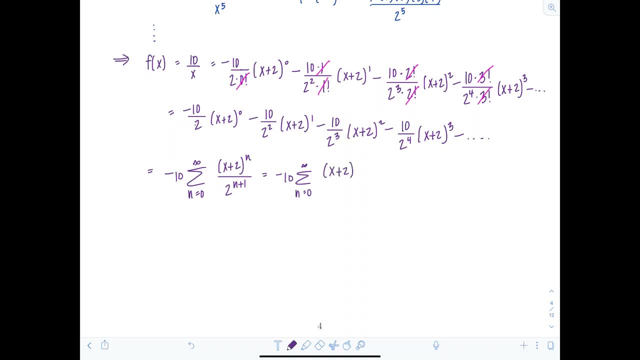 n equals 0 to infinity. We have x plus 2 to the n, over 2 to the first times, 2 to the n. So if you want to bring this negative 10 back inside the sum, negative 10 divided by 2 is: